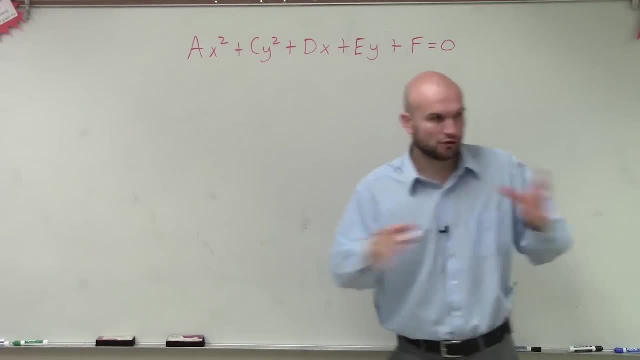 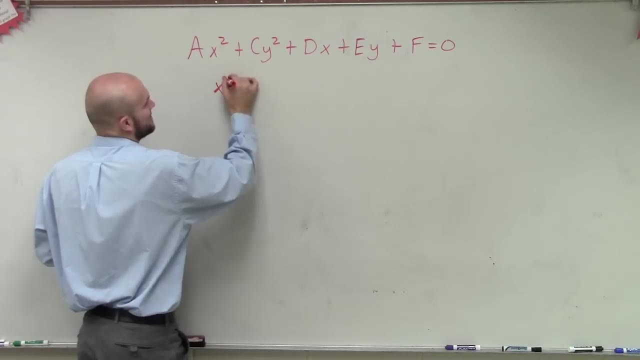 But we've also talked about standard forms, right, And I'm just going to go through one of them for each one, alright, and we'll kind of talk about it. So the first one we talked about was a parabola. When we said a parabola, we could rewrite as: x squared equal 4p. let's just do the x and k, that's fine. 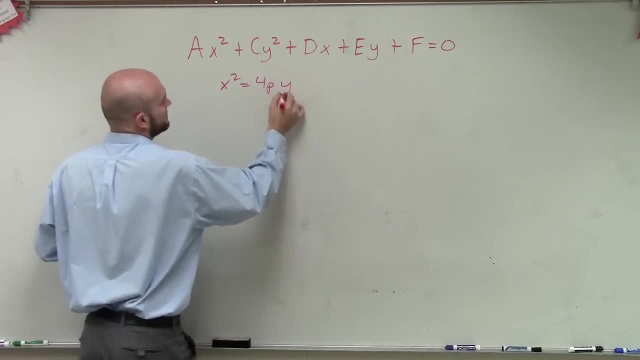 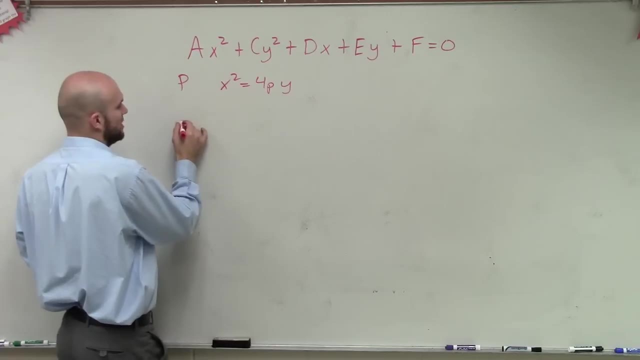 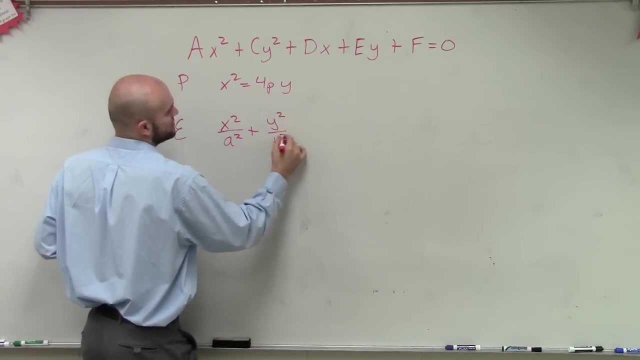 Actually, let's do so. x squared equals 4py. That is a parabola with the vertex at the origin right. So that was a parabola. then we talked about an ellipse, And remember ellipse had x squared over a squared, plus y squared over b, squared equals 1.. 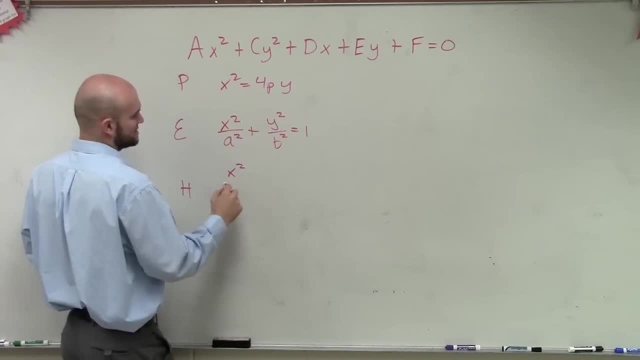 We had a hyperbola which was- let's just do this: x squared over a squared minus y squared over b squared equals 1.. And then we also talked about a circle, where a circle is going to be a special type of ellipse. 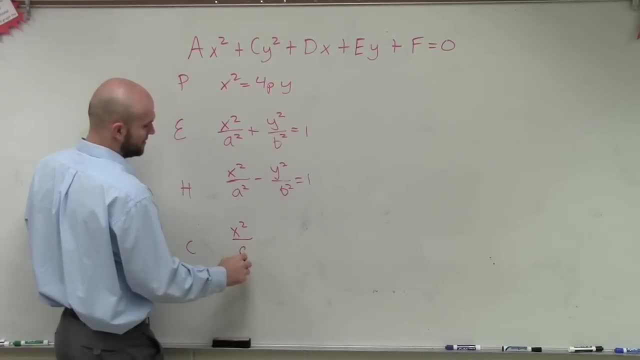 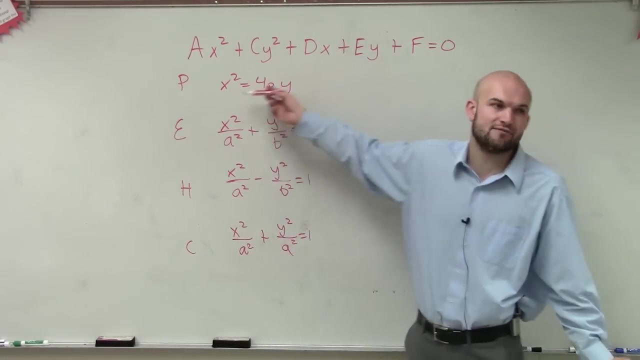 but a circle is when a and b are equal to each other, So we can just use a squared for each one. Now, ladies and gentlemen, for these three examples. alright, these are all hyperbolas, So some of these are verticals. actually, these all have a horizontal right. 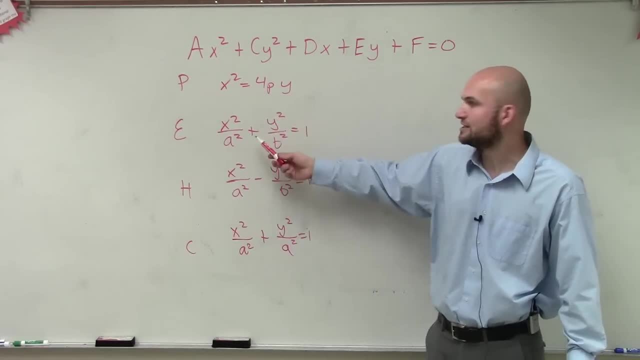 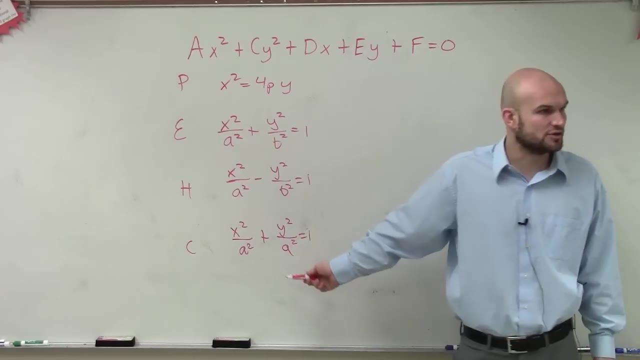 This is where I'm sorry. well, this one's going to be opening up and down. This one's where you're going to have a horizontal major axis. This will have a transverse axis which is horizontal, And this one is just going to be a circle. 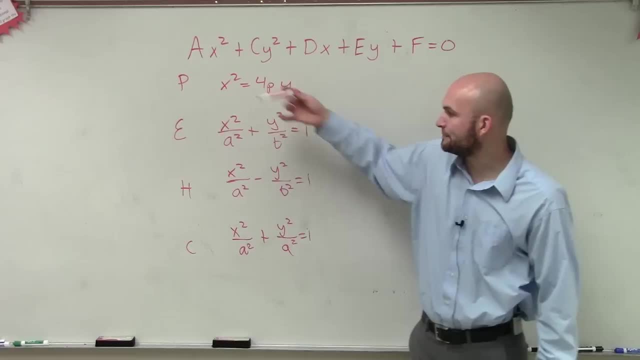 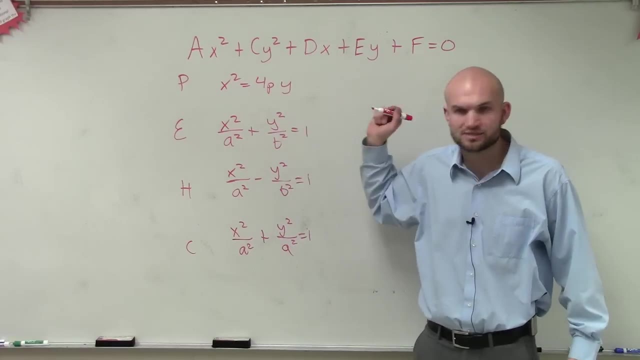 So this is just a little general form when I talk about parabola, ellipse, hyperbola and a circle. alright, Now, obviously you guys know there's another type of equation. right, You can have the equation where the parabola opens horizontally. 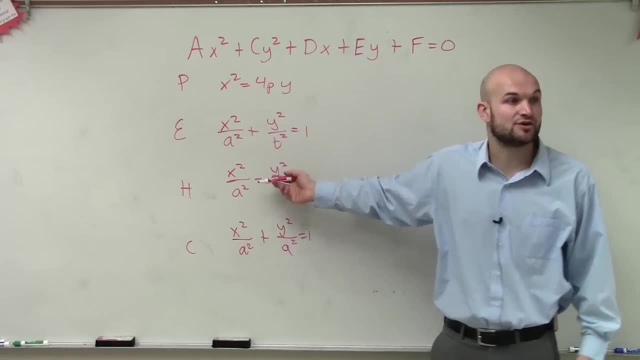 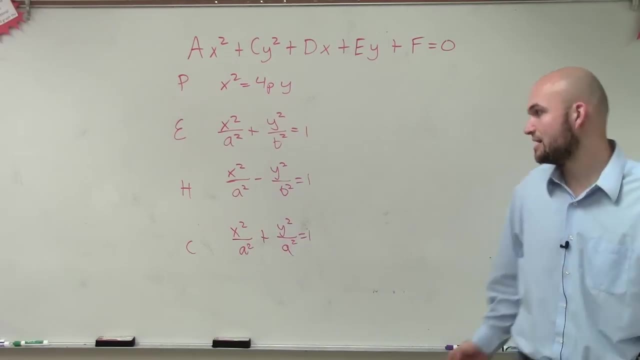 You can have a vertical major axis Here. you could have a transverse axis which is vertical, which would be the other formula. But the circle we notice is kind of always going to be the same. We always know that our a is going to equal each other, right? 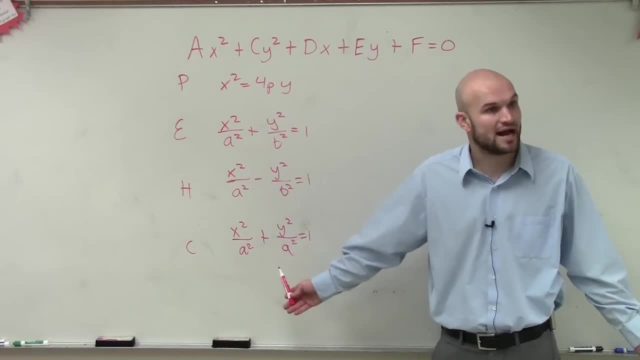 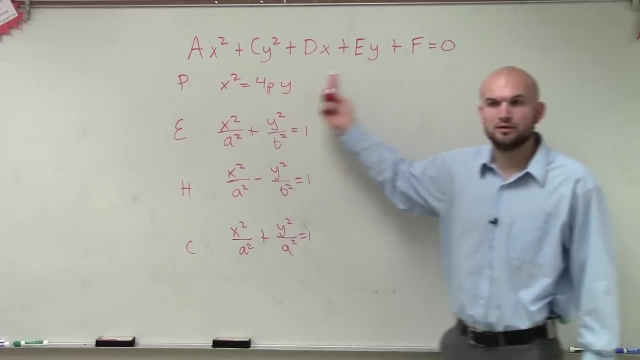 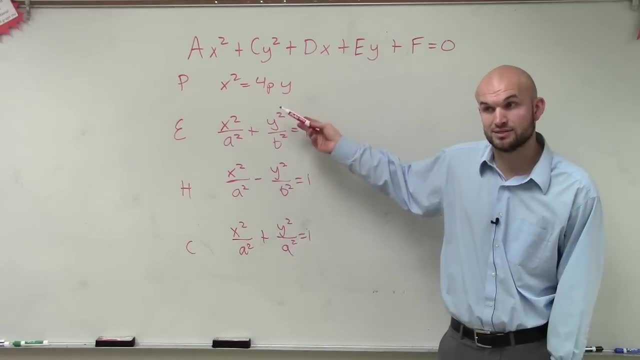 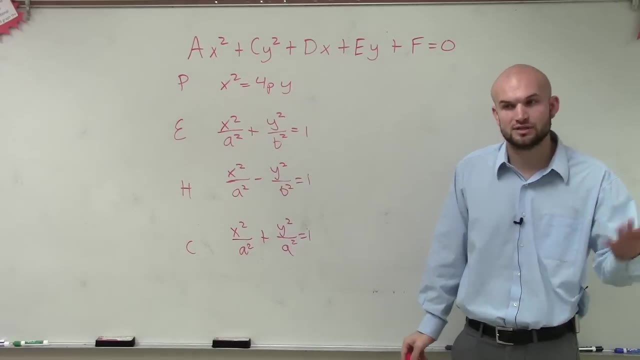 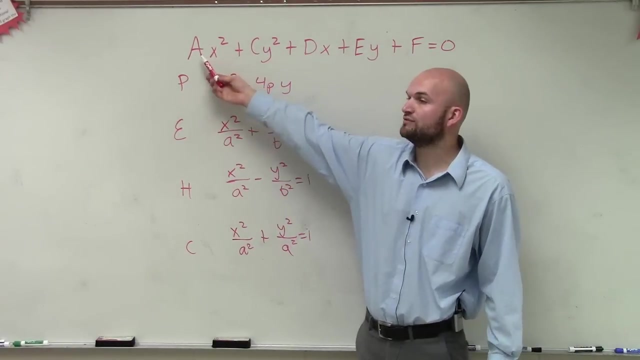 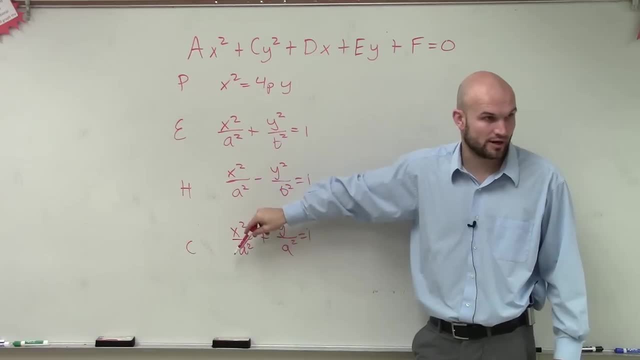 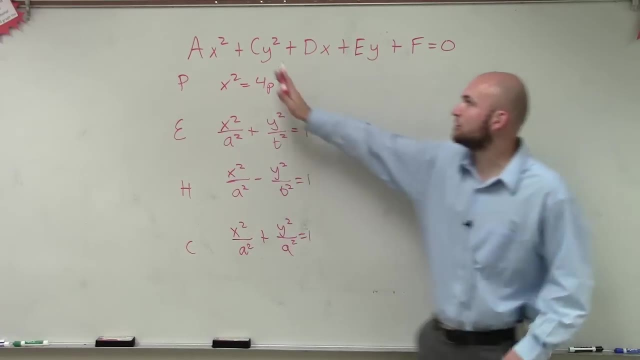 So what you guys notice is that really, our coefficient of x squared is 1 over a squared, And here for y is also going to be 1 over a squared. So, if you remember, what we can do is if the coefficients of my x squared and my y squared. 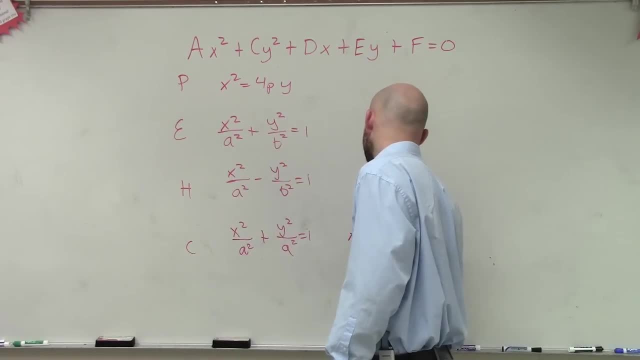 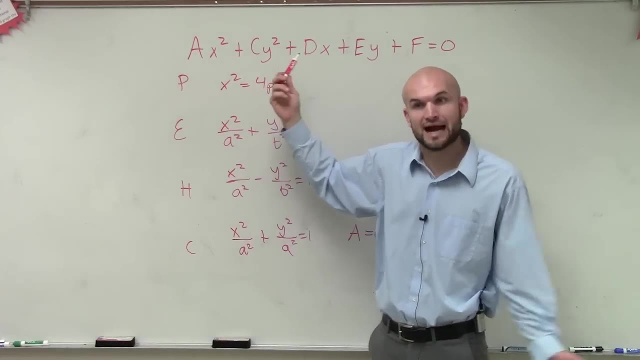 are exactly the same meaning. if a is equal to c, then you know you're going to have a circle. So if you look at an equation and you know a is equal to c, then obviously you know that your major axis and your minor 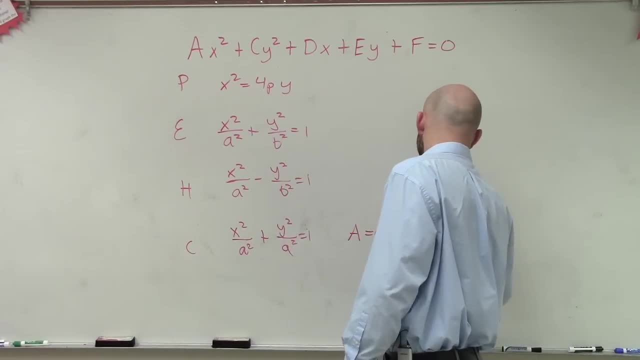 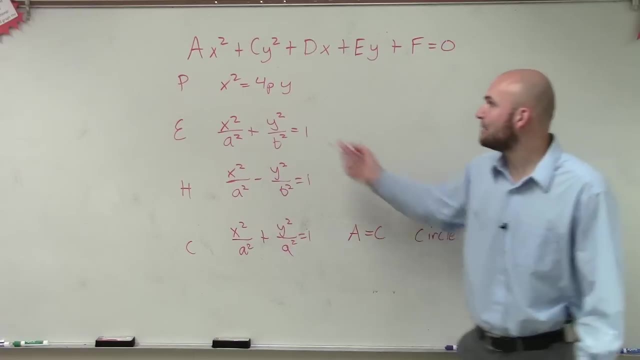 axis are the same. So if you have a equals c, that's going to tell you you have a circle. when you have a conic section written in this format, Let's look at a parabola. On a parabola, we only have 1 squared right. 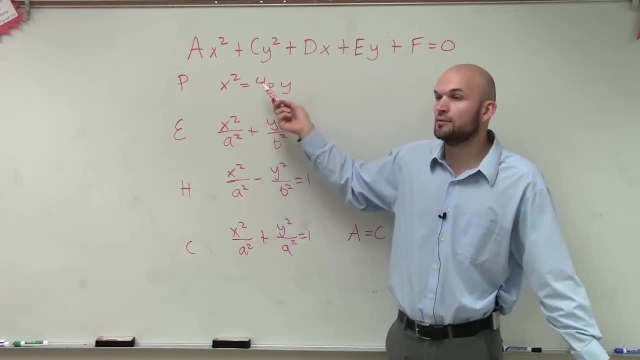 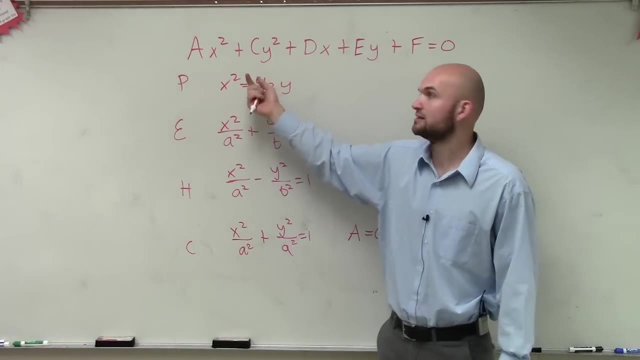 It's either x squared or y squared. In this case I have an x squared, So therefore I would have a 0 as the coefficient of y squared. So if we looked at, if I gave you a formula in this format, 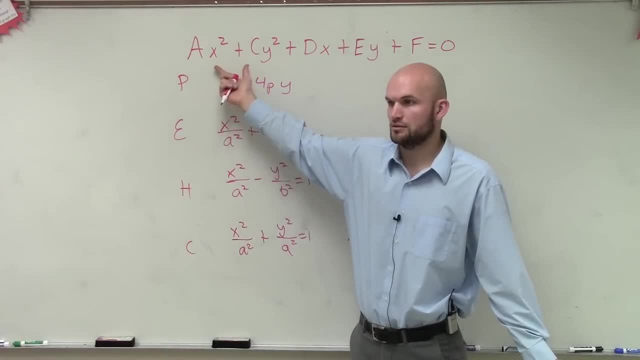 a or c, one of them would have to be 0,, correct? Yes, John, Correct, Only one of them has to be 0, because there's only 1 x squared or 1 y squared. So if you were to multiply a times c and you got 0,. 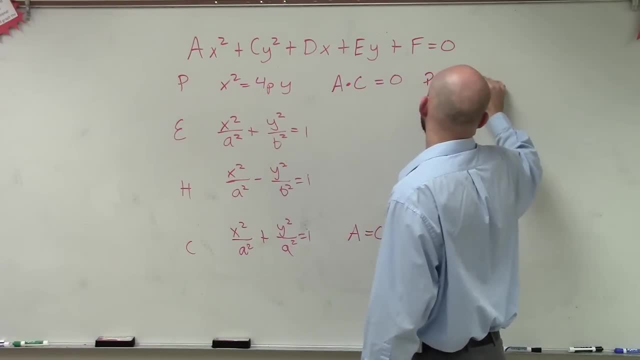 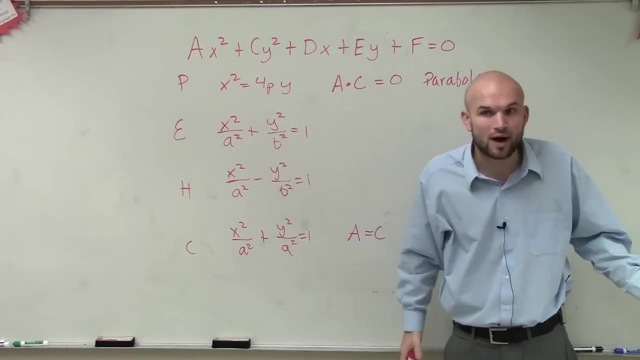 then you know you have a parabola. So what I would look at: if you're given a formula in this form, if you only have 1 x squared or 1 y squared, ladies and gentlemen, then you know you're going to have a parabola. 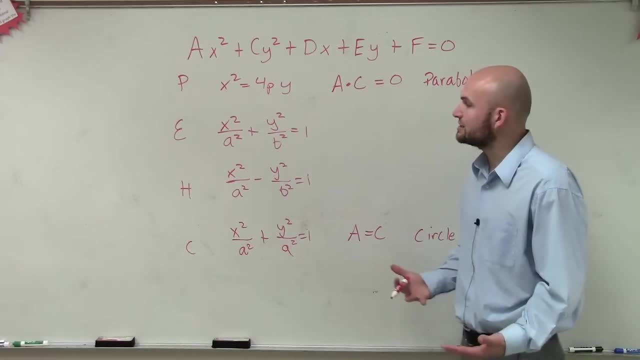 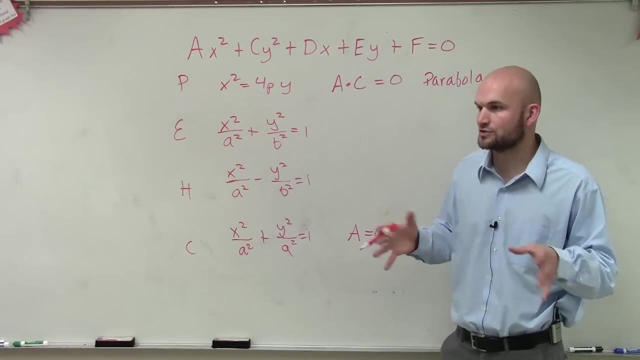 Now let's go and take a look at an ellipse and a hyperbola. Notice, ladies and gentlemen, that an ellipse we're always adding right. We're adding our x squared over 8, or we're adding the x squared and the y squared.